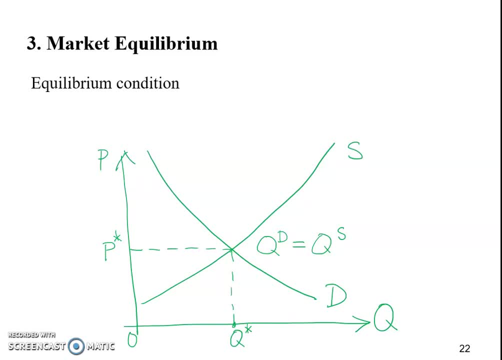 English means balance, means equivalent. the two sides are equal. so that's exactly what we are trying to say. you know, with this phrase: market equilibrium. sometimes you also heard people saying the market is clear at p-star. you also heard people saying the market is clear at p-star. 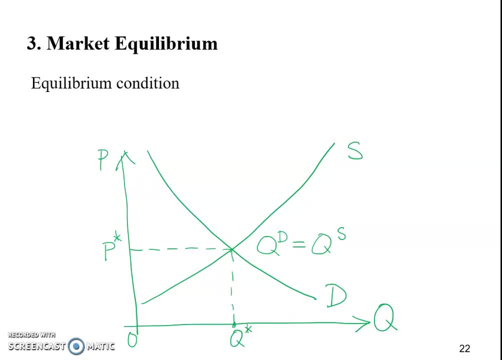 sometimes you also heard people saying: the market is clear at p-star again. that means nobody, you know, or everybody who wants to buy or sell would be able to do so. okay, at that specific price. nobody has been left over on the market and um, so the this one- QD equals QS- is the equilibrium condition, okay. 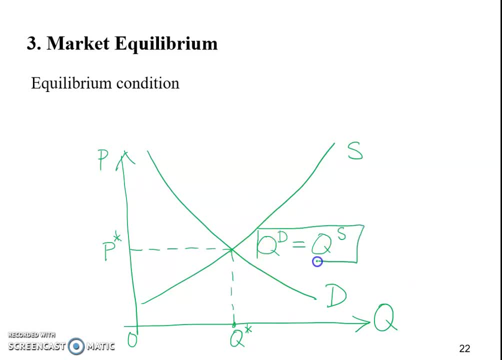 that's how we find where exactly the market equilibrium is. all right, and P star and Q star are equilibrium price and quantity respectively. okay, all right now. um, in reality, the economists won't believe that the market is always at the equilibrium, or the market is always clear, of course. now okay. 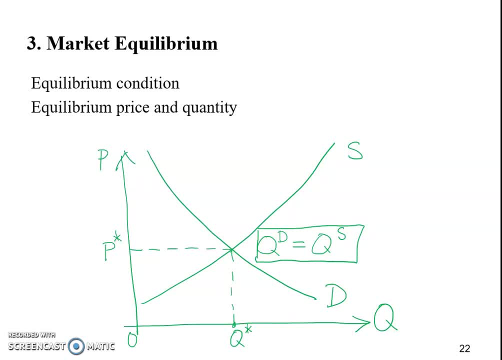 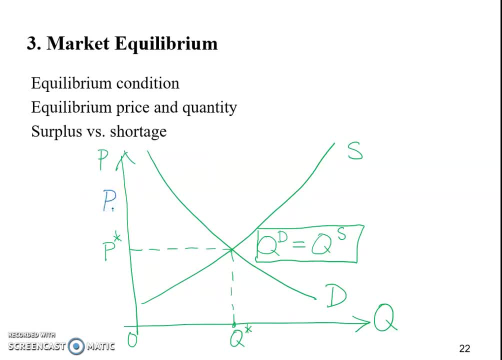 we're going to talk about that later. okay, now suppose, here again p1, it stays above the equivalent price. okay, now at p1 we find that, you know, if we go to the right and we hit the demand curve here, that means oops. sorry, this point stands for quantity demanded. okay, if we keep going to the 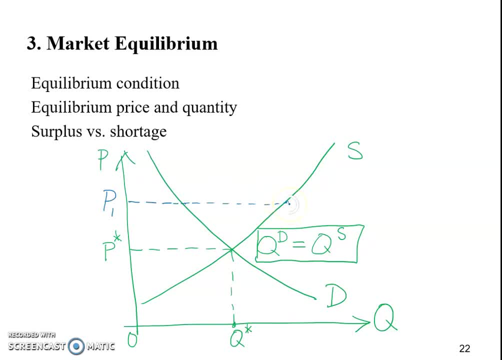 right, we find this point, that is, quantity supplied, because it's on the supply curve. okay, now we find a gap in between and this gap which tells us that, you know, the quantity of supply exceeds the quantity demanded. in other words, worry supply too much. okay, so this is so-called the surplus. 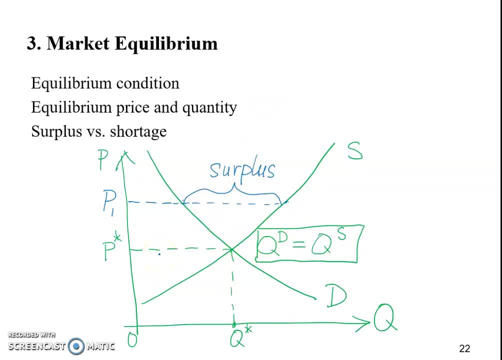 all right. and if surplus happens, then the centers or producers, if they already finish production- okay, for example, the restaurant already produced more pizza than what the market wants, okay, or leads- then what they could do at that moment is to lower the price. okay, once you know the price, you would. 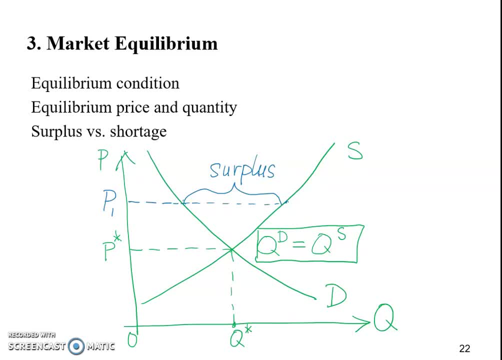 attract more buyers to buy pizza at your price. okay, when they start lowering the price, some restaurants would find that you know it's not worth producing pizza anymore, or it's not profitable anymore, so they're gonna quit, or some restaurants would reduce their pizza production. okay, so what we're gonna find is because the you know some firms on the market. 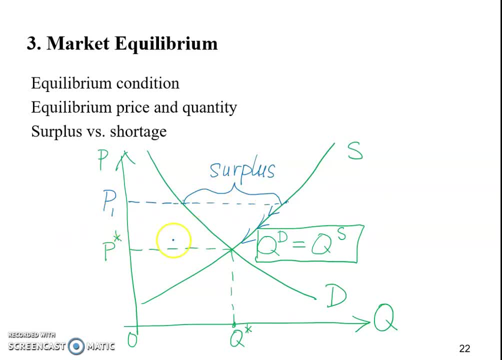 lowering their price, so the quantity supplied would be smaller. so we're moving down along the supply curve, okay, but remember, when the price is lower, the buyers on this market also find that right. so they believe that, you know. some of them believe that it's worth buying more pizza, right? or some of them used to buy hamburgers. 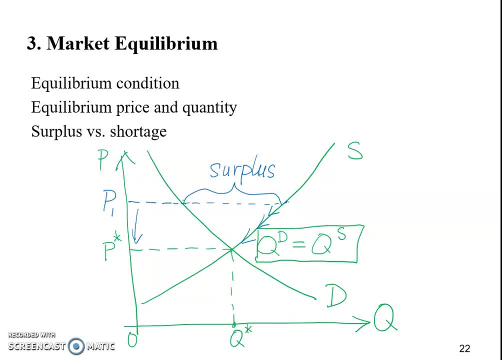 and or other types of food. now they find, you know, pizza becomes more affordable, so they want to switch to the purchase of pizza, right? so when people buy more, again, the quantity demanded increases. so we're moving along the curve, moving down along the curve. okay, again, this is a movement along the curve simply because it's caused by a change in the 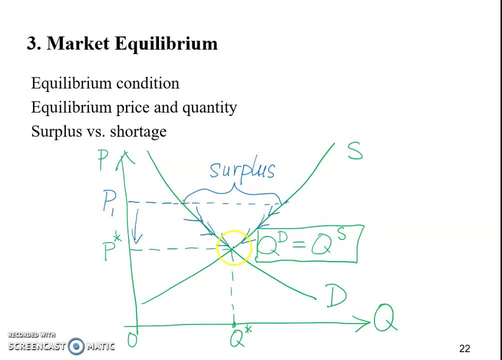 pizza price. okay, now you would find this movement will stop here, at the equilibrium point. okay, simply because at that point the sellers would have no more incentive to lower the price. okay, what they already produced can be sold on the market, all right. so, um, this is the case for surplus. okay, how we see, or where are we going to see, surplus, and 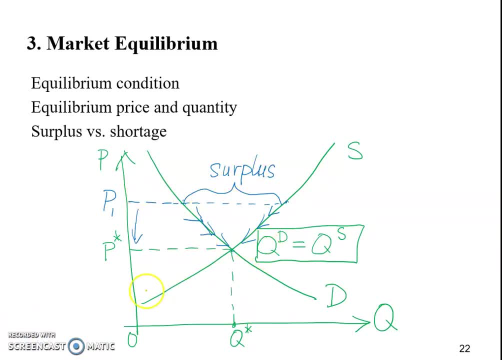 how the market by its own can eliminate the surplus. okay now the second case is: let's look at the price level lower than the equilibrium price. okay now, this time when we go to the right, we hit the supply curve first. so that point here on the curve. 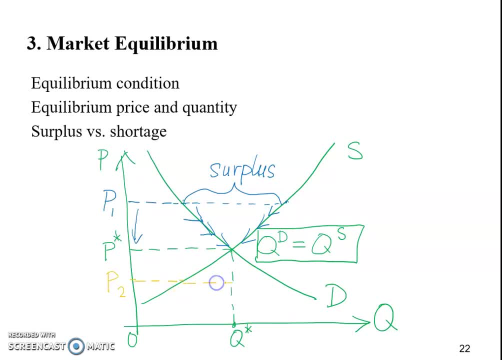 represents the quantity supplied. okay, if we keep going to the right and find the demand curve, so this is quantity demanded. okay, now, this gap in between is what we call shortage, because quantity demanded exceeds quantity supplied. okay, now, intuitively, this is pretty easy to understand. because the pizza is too cheap? okay, the price is too. 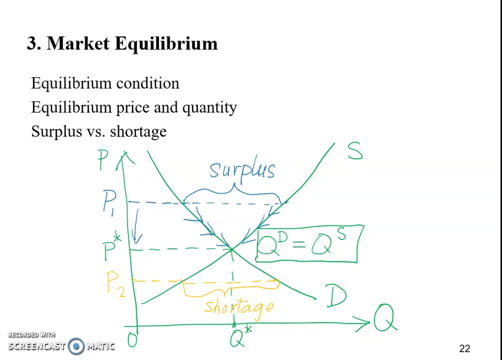 low. so we find a lot of people willing and able to buy it. but you know, on the supply side, the pizza makers find this is not profitable. okay, so they produce a significantly lower amount of pizzas. okay, now, if this happens, you know, if we see a shortage on the market, you would find that. 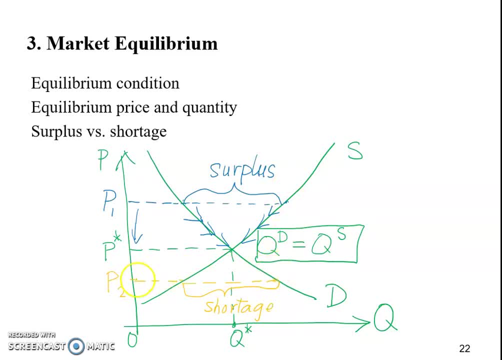 among the buyers, some of them will start beating up the price. okay, especially with these pizza lovers. they really enjoy pizza. they would like to offer a higher price to be sure they can get pizza- and remember there's not enough produced. so if they desperately want it, the best way to do that is to offer a higher price now, when more 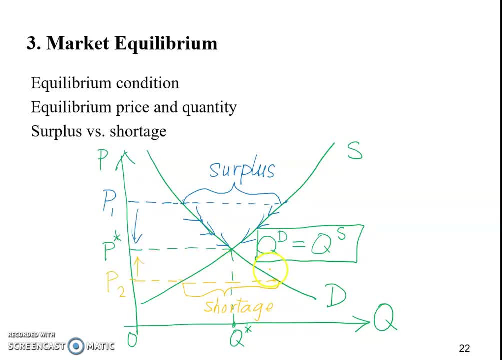 and more people are offering a higher price, then we're going to say that you know, quantity demanded reduce okay, so some people would stop purchasing pizza and buy other things like hamburgers, cheeseburgers, right, hot dogs. and when the quantity demanded decreases were moving up along the demand. 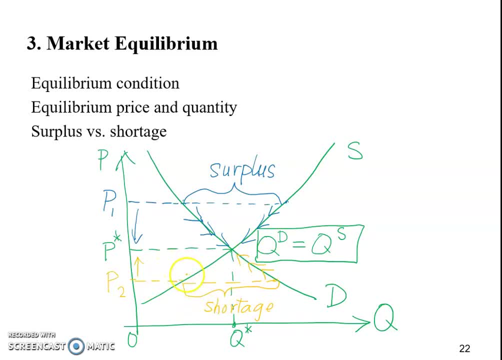 curve okay. now on the supply side, when the producers find that the price gets higher so it becomes more profitable producing pizza, they're going to come back and produce more crивается- okay. so that way the quantity supply will go up and we're moving up along the supply. 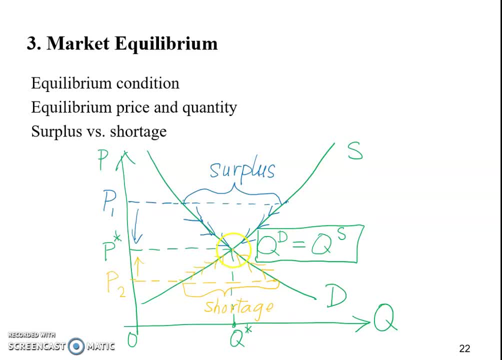 curve once again. eventually we will go back to this intersection, the equilibrium point. okay, so the point we want to get across here is: um, sometimes people say you know the economist? um, We believe the market is always at the equilibrium, The market is always clear. That is the misunderstanding. We come up with the equilibrium condition or the market equilibrium. 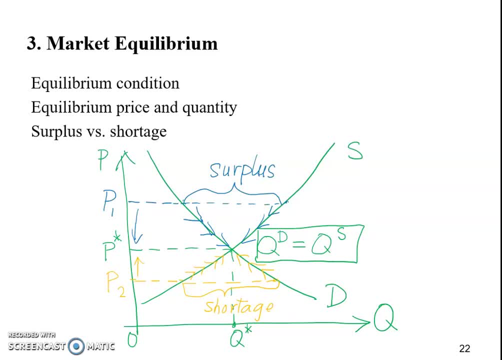 not because we really believe the market is always going to be there. We use the equilibrium condition as a benchmark so that we can talk about the surplus and shortage. What's more interesting to us is we believe the market by its own can eliminate the surplus or shortage in the long run. 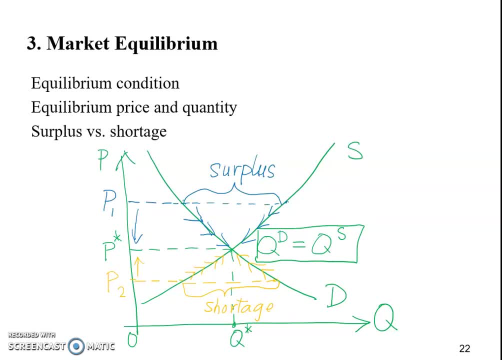 So in the short run we might see some deviations from the equilibrium, But in the long run we believe this is actually a pretty stable situation. So, for example, when the price happens to be higher, like P1 here on the graph, and we are going to see a surplus,